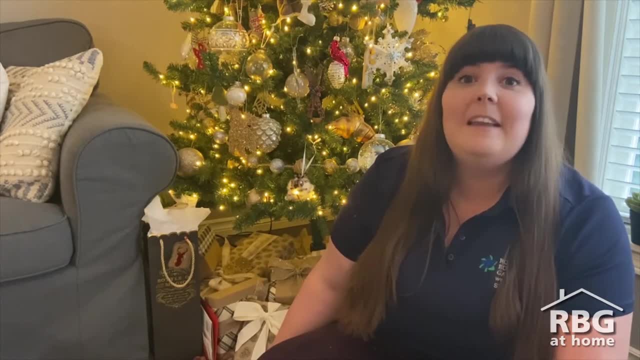 our crafts together. for us, We do have to use a little bit in order to hold them together, but we're using as little plastic as possible. While I recommend using hot glue, as it does dry, you get instant results. it is hot, so you may need help from a big person. 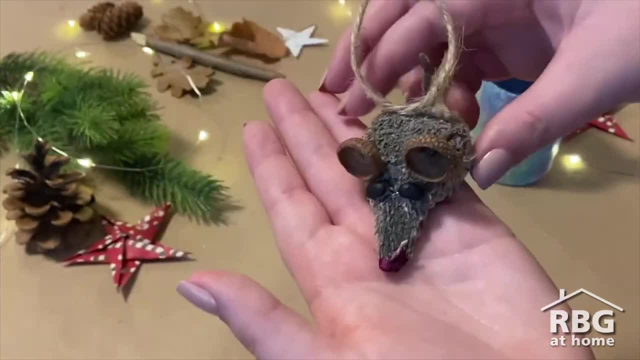 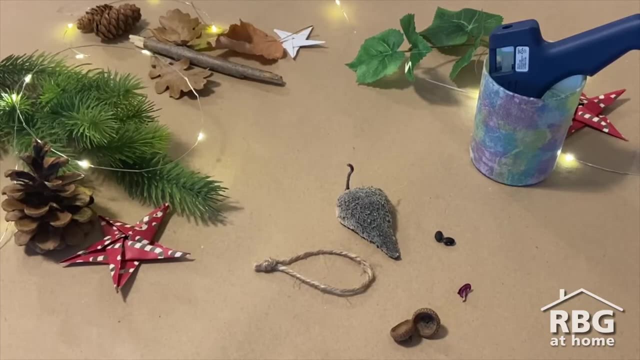 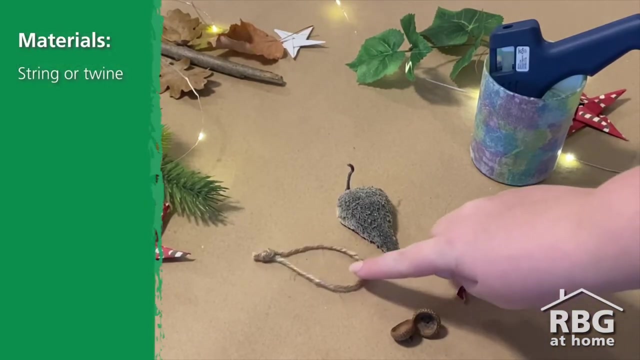 Today, we're going to make a pinecone owl as well as a milkweed mouse. Let's get started. So the first craft that we're going to make today is a milkweed mouse. There are five different things that you need in order to make this craft: A piece of twine- I've pre-tied this one. 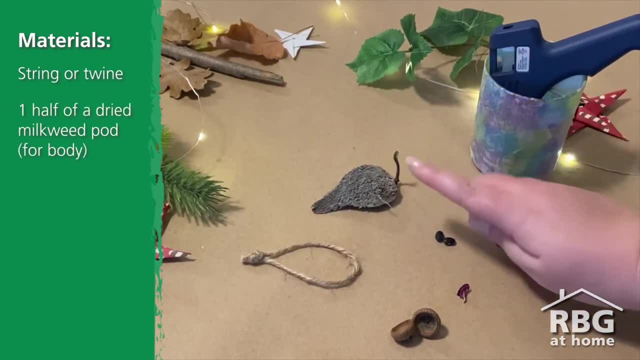 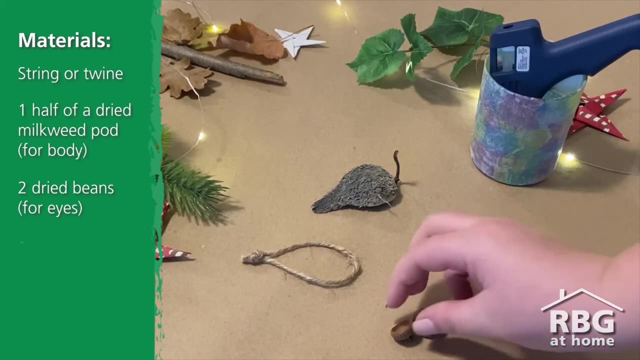 A milkweed pod, and it's really helpful if the stem is still attached, since it makes a tail. Two dried black beans to be your eyes, two acorns to be your ears, and I have a dried flower for his nose. So let's get started. 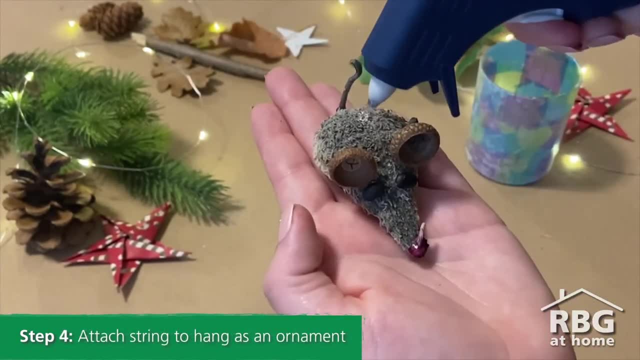 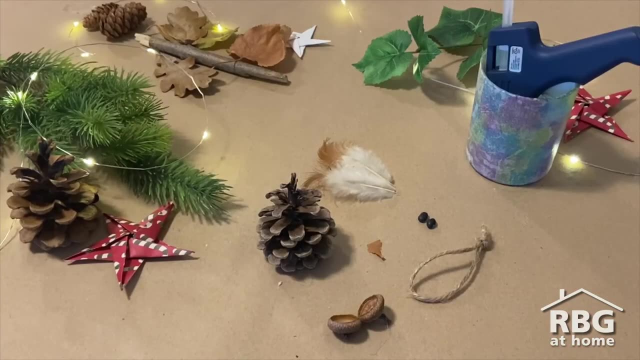 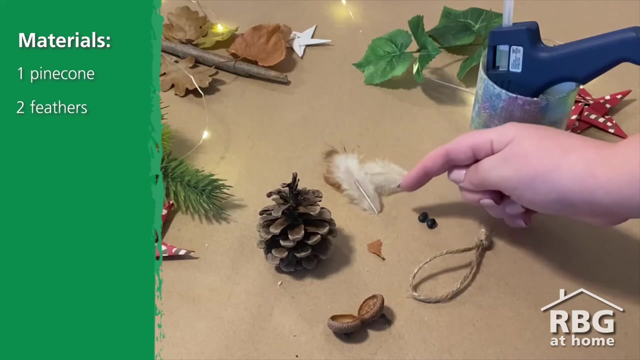 So for our next craft, we're going to make an owl. There's six things that you need in this craft: A pinecone, two feathers, a nose of some sort- I'm using a piece of a dried leaf- Two dried black beans for your eyes, two acorn caps, also for your eyes. 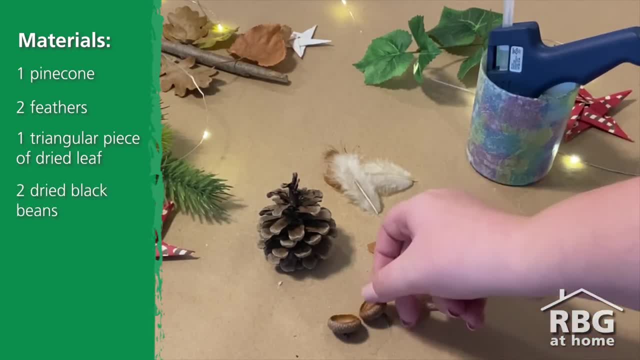 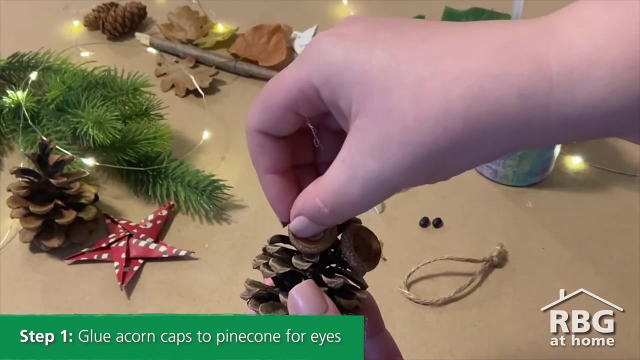 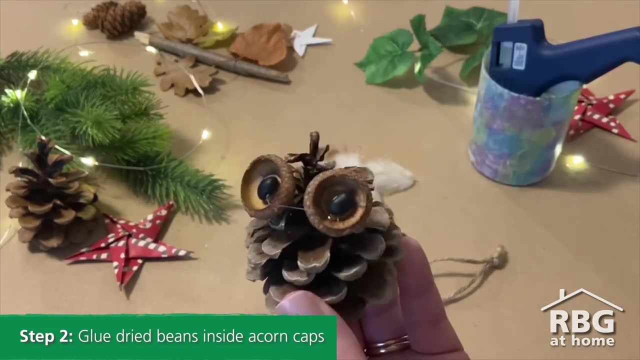 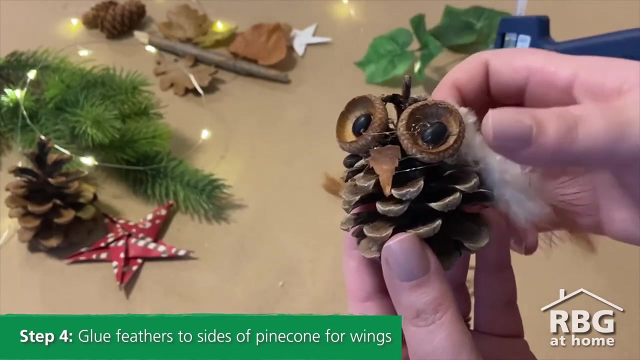 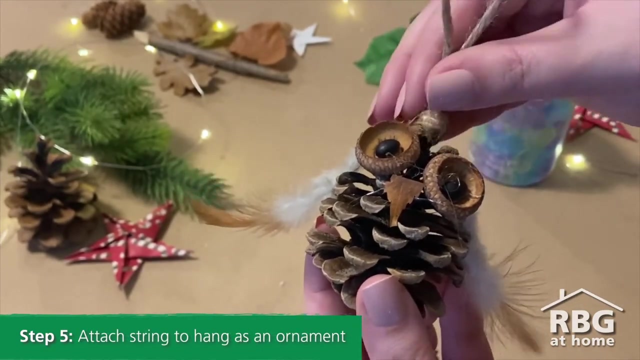 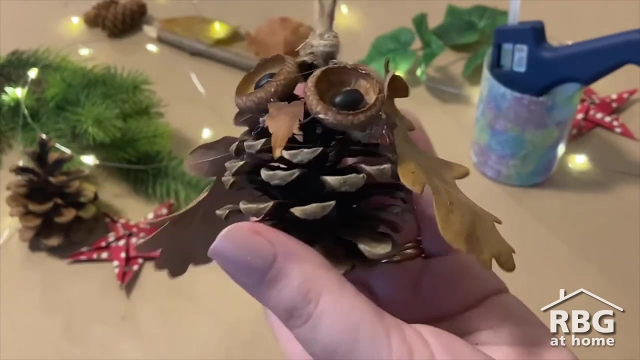 and some dry leaves. Two eyes for him, Two eyes for me, Two eyes for him and a piece of twine to add your owl to your tree. Now, if you don't have feathers available to you, you could actually use dried leaves as your wing. 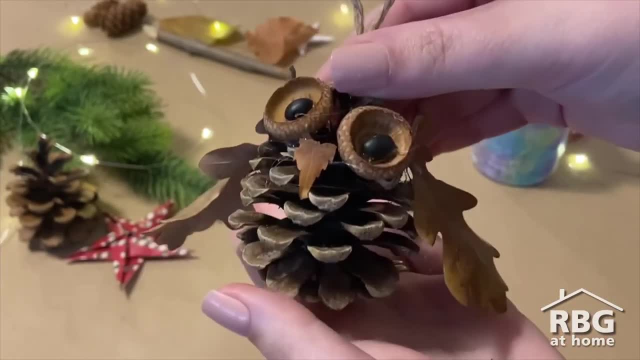 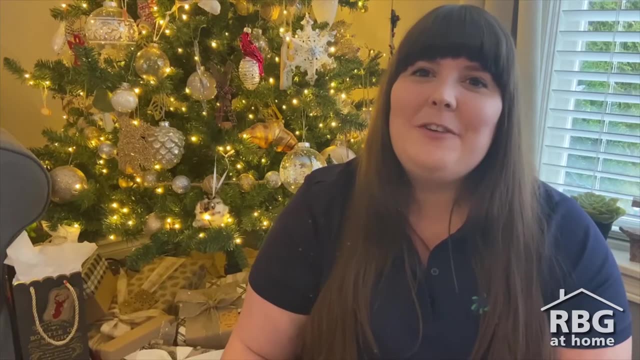 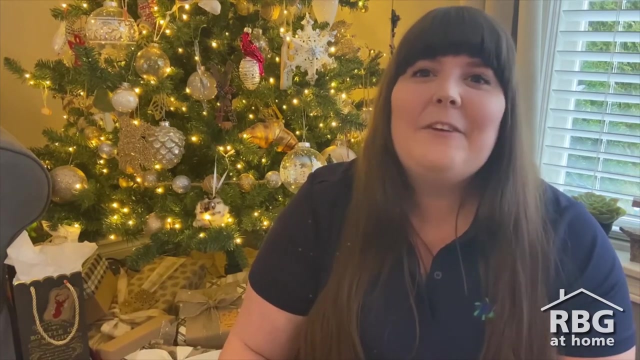 So here I've used two oak leaves to make my little owl friend, without finding feathers. I hope you enjoyed making these cute owls and mice with me today. or maybe you created a creature all on your own invention. Let your creative juices flow.